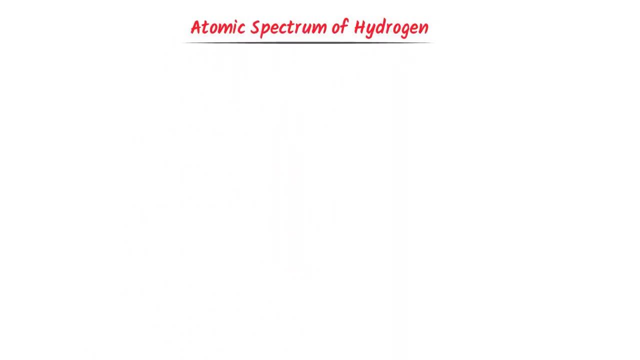 Atomic spectrum of hydrogen. Firstly, we will learn some key concepts like spectrum. Consider sunlight: We know that when we pass sunlight from a prism, different wavelengths bend at different angles or we get seven different colors. Remember that these different colors represent different radiations or different wavelengths. We call this group of radiations. 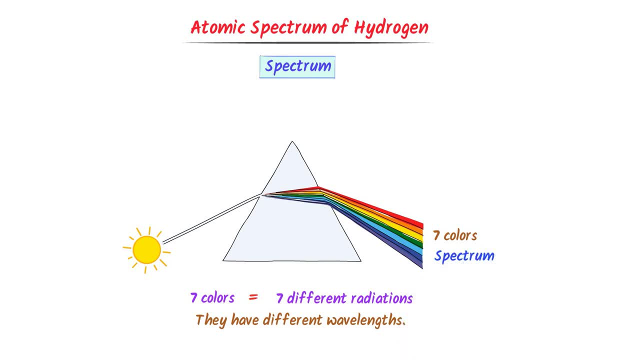 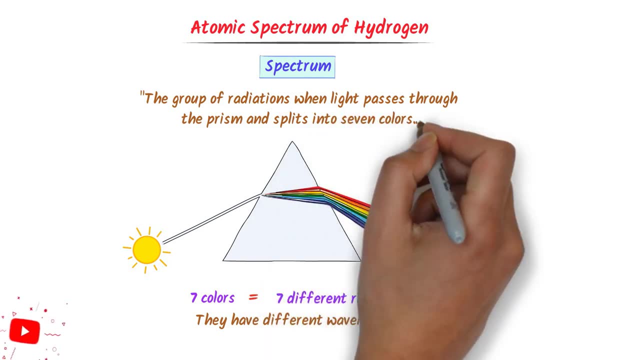 or wavelengths as spectrum. Therefore we define spectrum as the group of radiations. when light passes through the prism and splits into seven colors is called spectrum. Just remember that spectrum is a group of radiations. Now we will learn types of spectrum There. 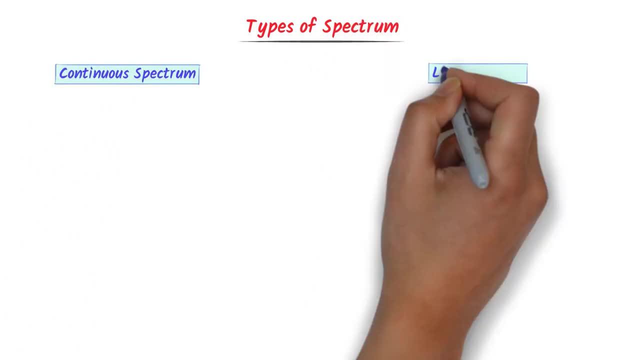 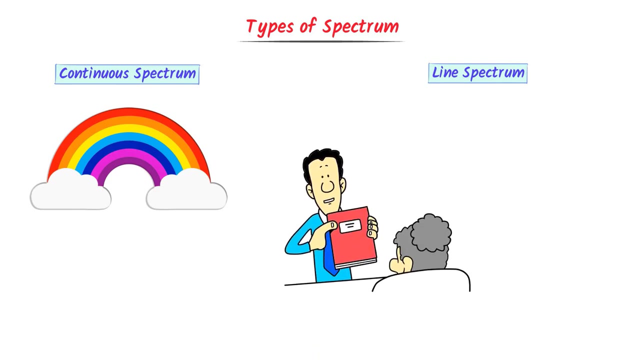 are two types of spectrum: continuous spectrum and line spectrum. In case of continuous spectrum, continuous spectrum can be defined as a group of radiations. Now we will learn types of spectrum. Consider this rainbow. Now. I always teach these three very important points about. 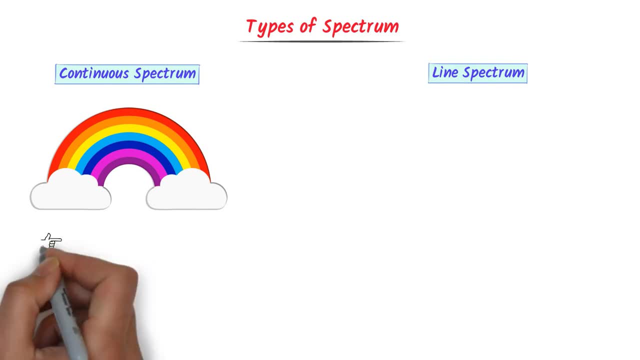 continuous spectrum. We can see that rainbow has no clear boundary line between colors. Secondly, the colors of rainbow partially overlap upon each other. Thirdly, the colors of rainbow is not separated by lines. Remember that such type of spectrum is called as continuous. 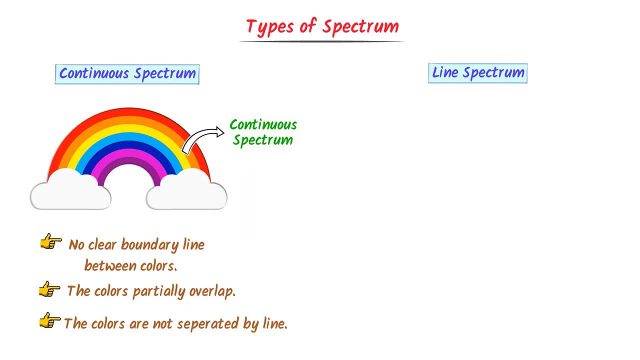 spectrum Because all the colors are present in a continuous way. So whenever you listen continuous spectrum, always remind this rainbow. Now, what about the line spectrum? Well, personally I call it discontinuous spectrum, because it helps my students to remember this concept easily. 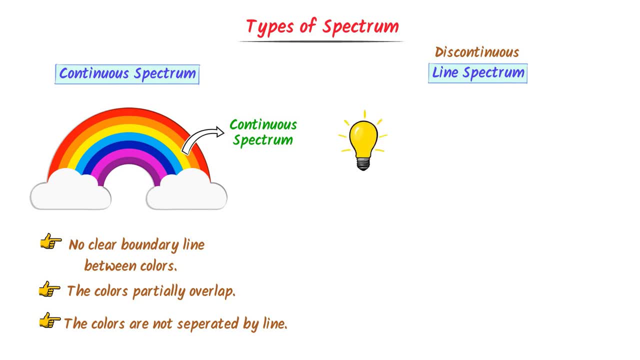 Let's consider this fluorescent lamp. When we pass its light through the prism, we get only these colors. I mean, we only get these colors. we only get four colors. I also teach three very important points about line spectrum. We can see clear boundary lines between colors. Secondly, these colors do not overlap upon. 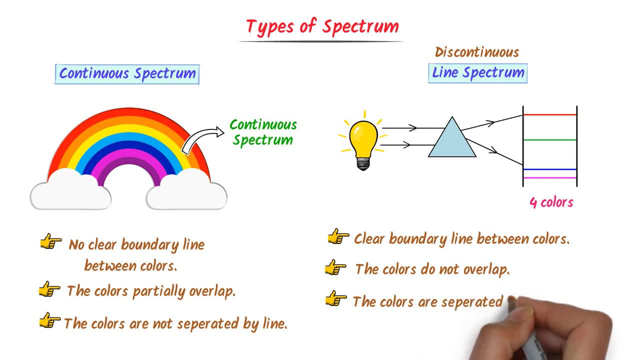 each other. Thirdly, these colors are separated from one another. Remember that such type of spectrum is called line spectrum, Because in this spectrum we only get lines. Personally, I call it discontinue spectrum, because this spectrum is discontinued in between. Hence, 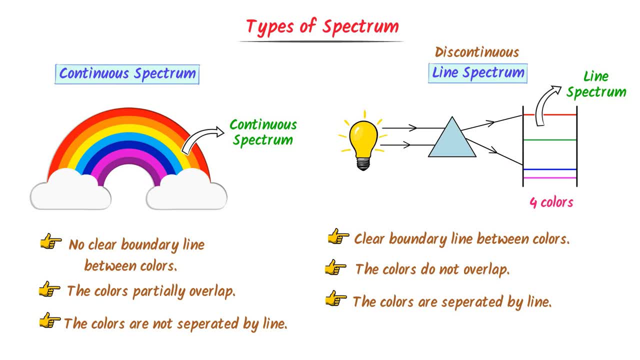 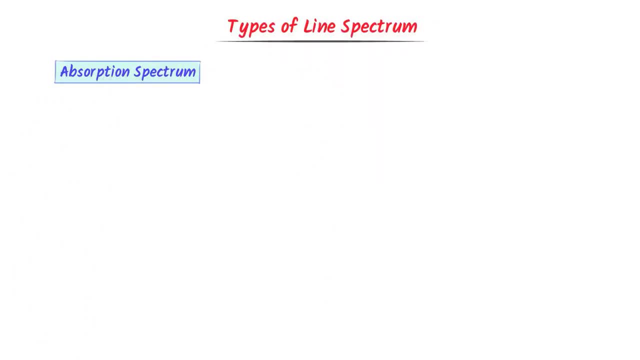 whenever you listen line spectrum, always remember this spectrum of fluorescent lamp. Now there are two types of line spectrum, like line absorption spectrum and line emission spectrum. It is very difficult topic for the students and I will teach this difficult topic in my personal way. 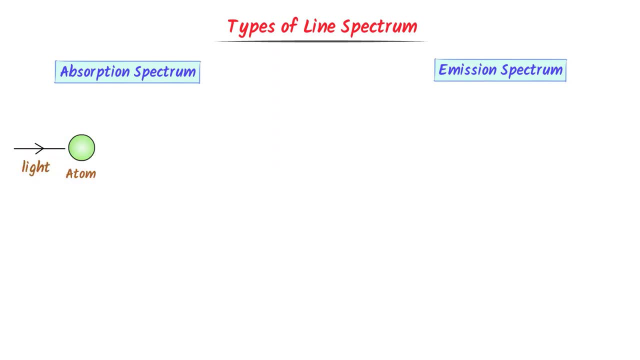 Consider this atom. Let white light falls on this atom. It will absorb some radiations from white light and will emit the remaining radiations. Now I pass these emitted radiation through the prism and I trace these radiations on the screen. We can see that some colors. 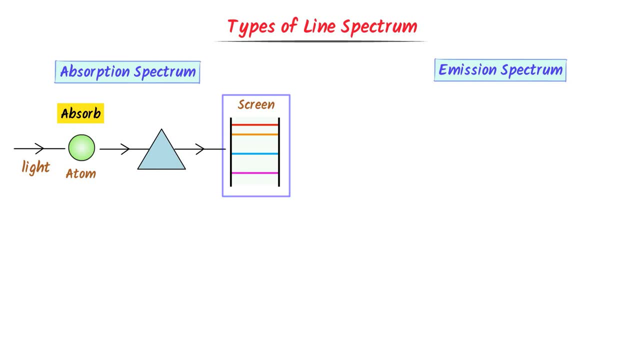 are missing in this spectrum? I mean, I only get four colors and three colors are missing. spectrum of white light. Can you guess that? why these 3 colors are missing? Well, this atom has absorbed 3 colors or 3 radiations from the 7 colors. We call this line spectrum. 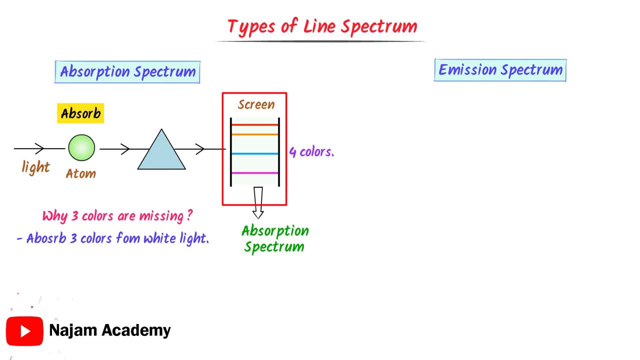 as absorption spectrum because this atom absorbs 3 colors. Let me repeat it: We call this line spectrum as absorption spectrum because this atom absorbs 3 colors. Hence, absorption spectrum is the one in which atom absorbs specific colors or specific wavelengths. On the other, 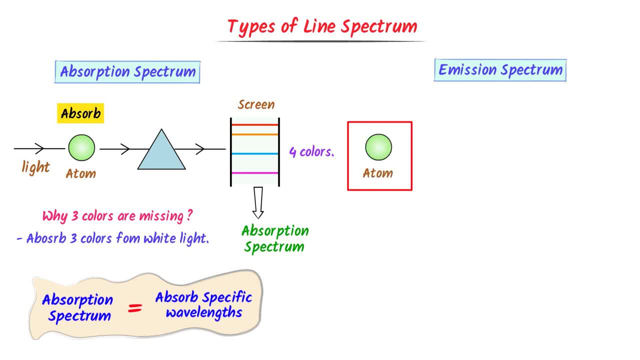 hand, this atom will cool down after some time. As a result, it emits all the 3 colors which it absorbed from the white light. I pass these radiations through the prism and trace them to the white light. I pass these radiations through the prism and trace them. 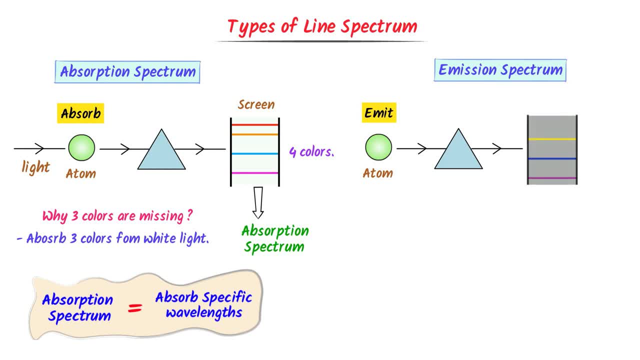 on the screen We can see that we only get 3 lines or 3 colors, Or we say that we get 3 wavelengths on the black screen. We call this line spectrum as emission spectrum because this atom emits 3 colors. Let me repeat it: We call this line spectrum as emission spectrum. 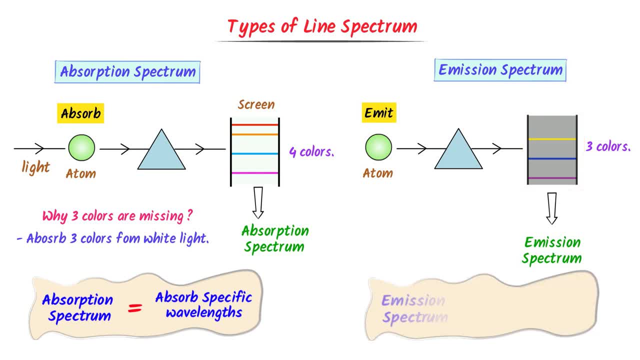 because this atom emits 3 colors. Hence, emission spectrum is the one in which atom emits specific colors or specific wavelengths. Thus, note down all these important points. Now I will give you a deep dive in order to learn this concept at advanced level. Firstly, we will 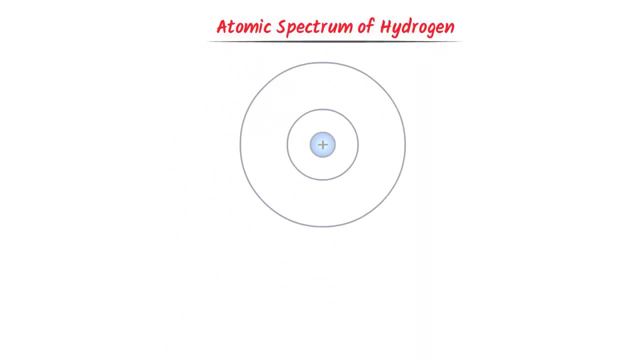 learn atomic spectrum of hydrogen. Consider this atom at ground state. We provide some sort of energy to this atom. According to Bohr-Baba, this electron in the first energy level will absorb this energy and the second energy level will absorb this energy and the 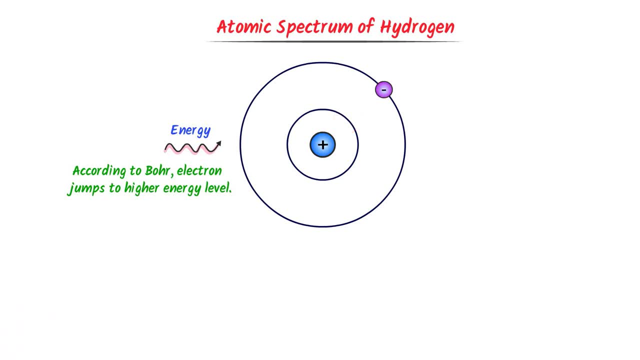 and it will jump to higher energy level. After some time, this electron will lose its energy in the form of radiation. Let me repeat it: After some time, this electron will lose its energy in the form of radiation. As a result, it will jump back to lower energy level. 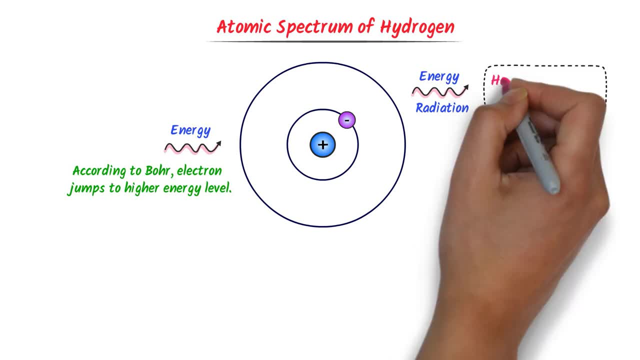 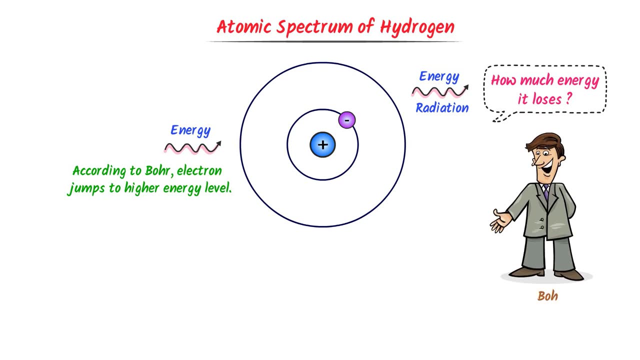 Now here is one very, very important question: How much energy this electron loses when it jumps back? Well, this question is answered by Bohr Baba. He states that the energy emitted by the electron in the form of radiation is equal to the energy difference. 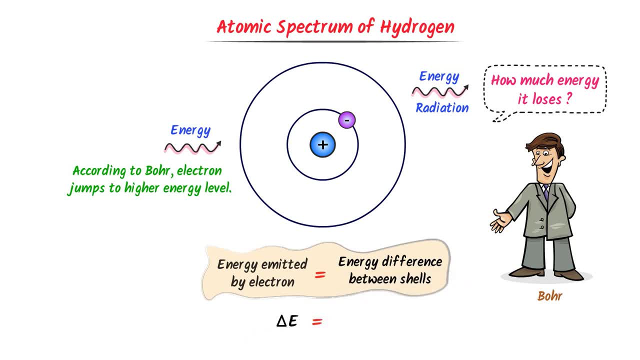 between the levels r del E is equal to E2 minus E1.. To conclude this whole concept, we learn that when an electron jumps from high energy level to low energy level, electron emit energy in the form of electromagnetic radiations. Hence noted down this fundamental concept of spectroscopy. 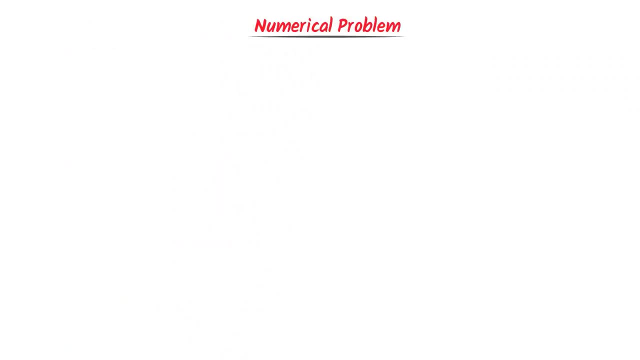 Now consider this numerical problem, which will further clear your concept. An electron of hydrogen jumped from n is equal to 2 energy level to n is equal to 1 energy level. Find the energy emitted by the electron. Well, according to Bohr Baba, 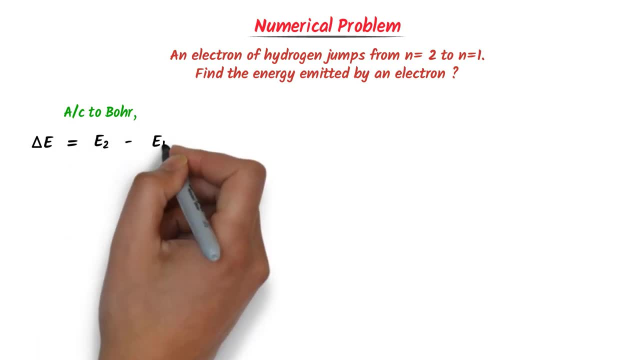 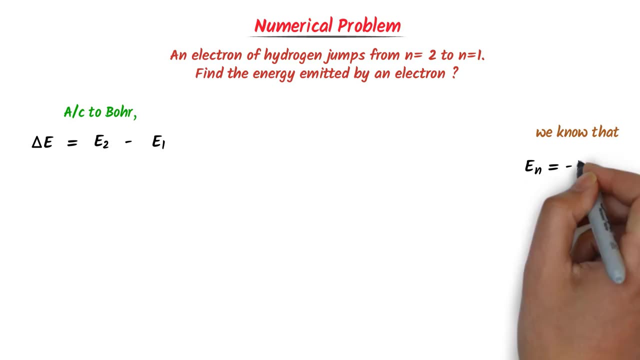 this energy del E is equal to E2 minus E1.. We know that the energy of nth level is equal to minus 13.6 z squared upon n squared. Now I write: del E is equal to minus 13.6 z squared upon n squared. 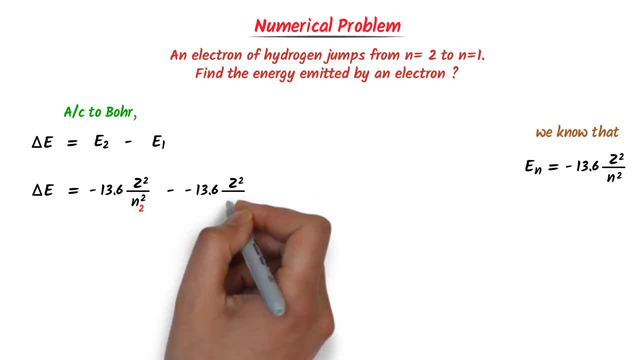 minus minus 13.6 z squared upon n squared. Or I write: del E is equal to this minus into this minus is equal to positive: 13.6 z squared upon n squared, minus 13.6 z squared upon n squared. Now I take 13.6 z squared as common. 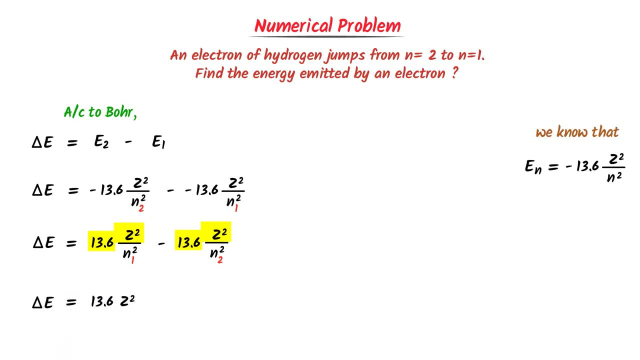 del E is equal to 13.6 z squared into 1 upon n1 squared, minus 1 upon n2 squared, We know that the atomic number of hydrogen, z, is equal to 1.. I write: del E is equal to 13.6 into 1 squared. 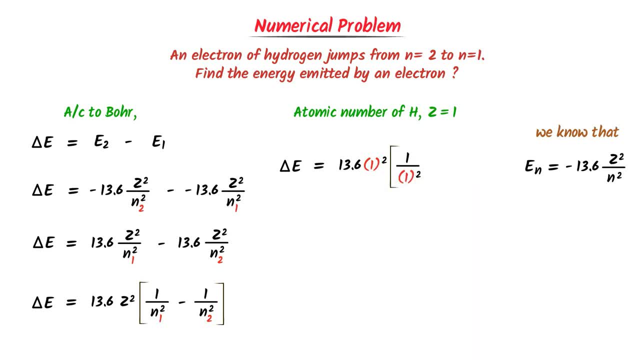 into 1 upon 1 squared minus 1 upon 2 squared. After calculation I get 10.2 electron volt. Hence electron will lose 10.2 electron volt energy when it jumps from second energy level to first energy level. 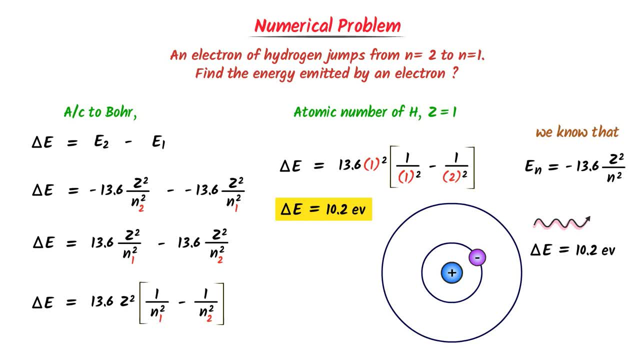 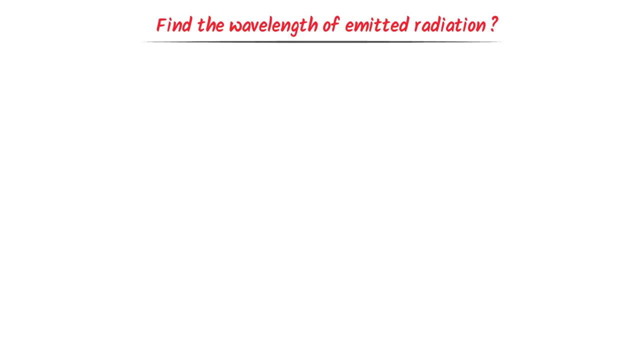 So note it down, this important numerical problem. Now here is the most important question of this lecture: How can we find the wavelength of emitted radiation? Well, to find it, consider this example: I take this atom. I provide some sort of heat to it. 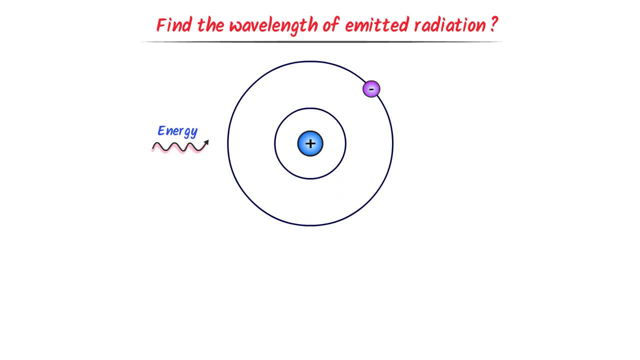 The electron absorbs the given energy and jumps from lower energy level to high energy level. After some time, this electron will lose energy in the form of radiations. My question is that how can we find the wavelength of this radiation? Well, we know that. 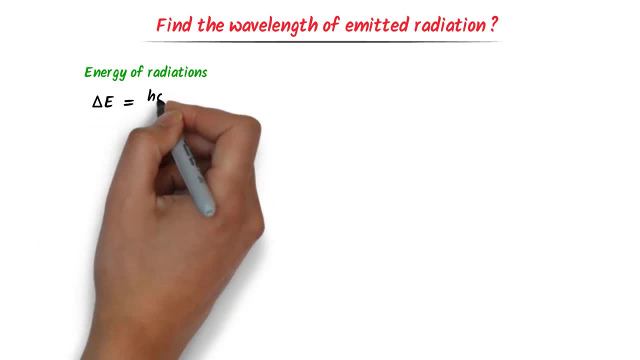 energy of radiation is equal to hc upon lambda. Let this is equation number 1.. Secondly, we know that the energy difference between shells is equal to e2 minus e1.. Let this is equation number 2.. Now comparing, equation number 1. 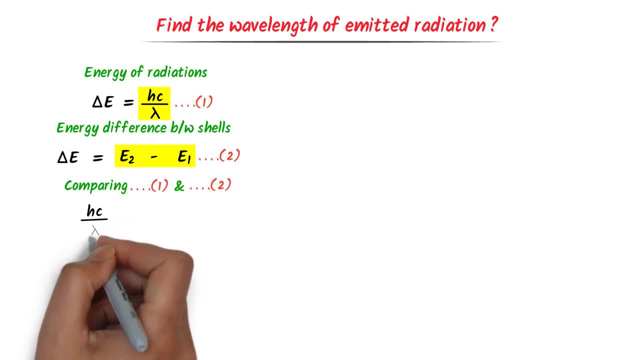 and equation number 2, we get: hc upon lambda is equal to e2 minus e1.. We know that the energy of nth shell is minus 13.6 z squared upon n squared. I write, hc upon lambda is equal to minus 13.6 z squared. 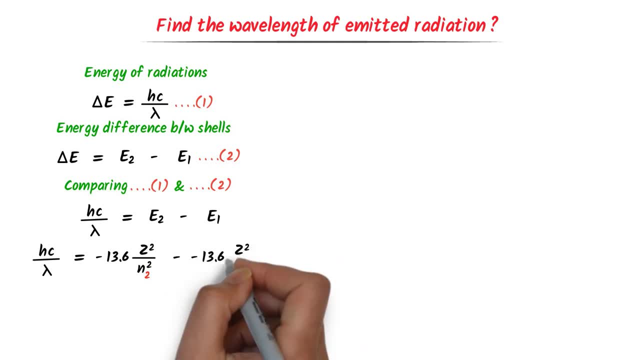 upon n2 squared, minus minus 13.6 z squared upon n1 squared, This minus and this minus becomes plus, I get. hc is equal to 13.6 z squared upon n1 squared, minus 13.6 z squared upon n2 squared. 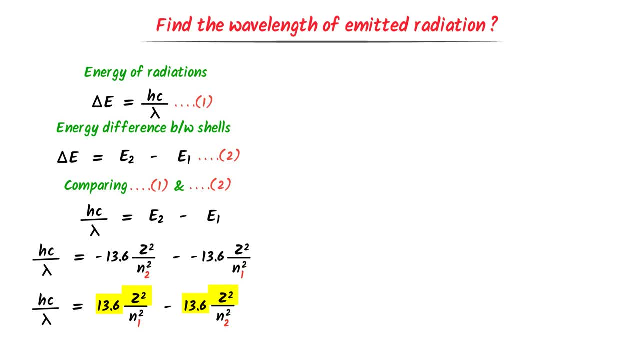 I take this 13.6 z squared as common. I get 13.6 z squared into 1 upon n1 squared minus 1 upon n2 squared. I bring this hc from the left hand side to the right hand side. I get. 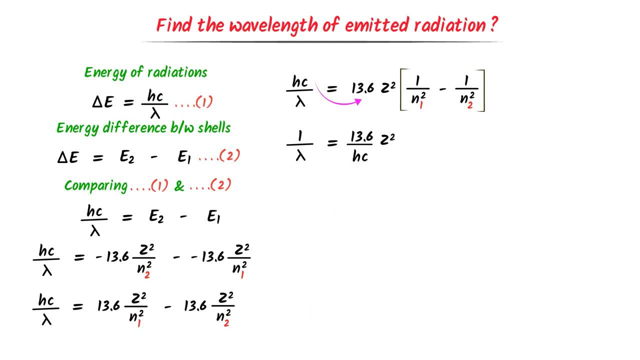 1 upon lambda is equal to 13.6 upon hc. z squared into 1 upon n1 squared minus 1 upon n2 squared Here, 13.6 upon hc is equal to r. We call this Redberg's constant. 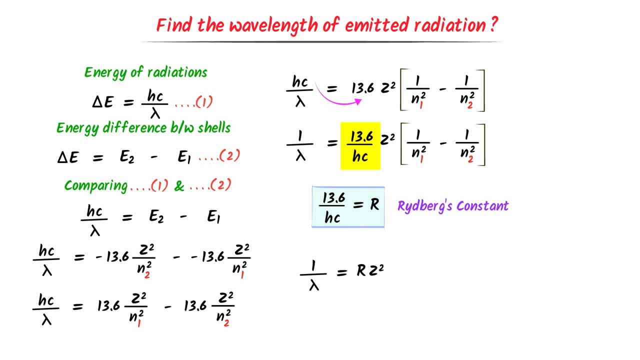 I get. 1 upon lambda is equal to rg squared into 1 upon n1 squared, minus 1 upon n2 squared. Thus, using this equation, we can easily find the value of any wavelength. Hence, remember this important equation Here, remember this important point. 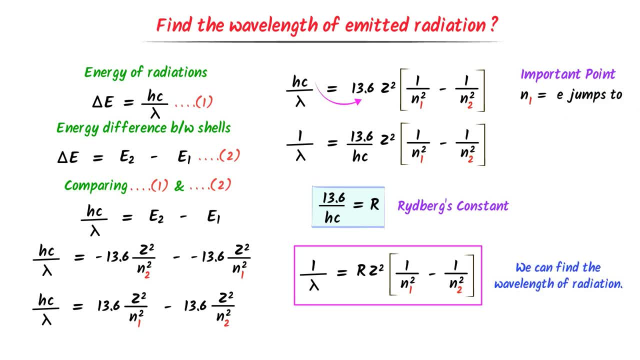 n1 is the energy level where electron jumps to, while n2 is the energy level where electron jumps from. Secondly, I use this trick to remember this equation: 1 upon lambda is equal to rate of zebra, is 1 by 9 minus 1 by 9.. 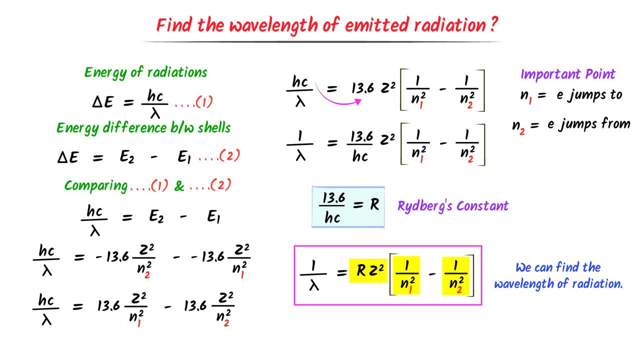 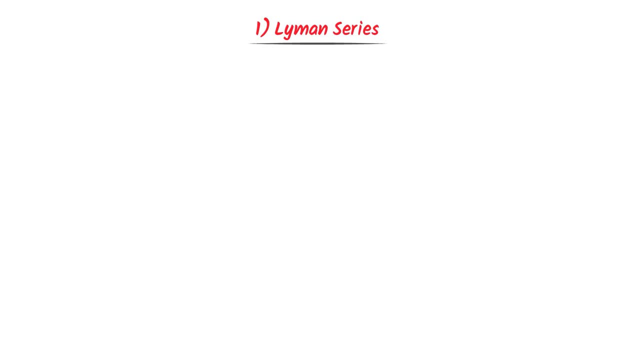 It easily reminds me this whole equation. Hence note it down. all these important points. Now we will learn the different series of atomic spectrum of hydrogen. The first one is Lyman series. Remember these two points about Lyman series. Firstly, 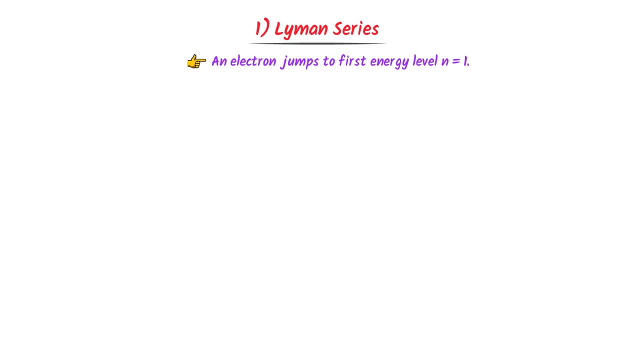 an electron jumps to first energy level. n is equal to 1 in Lyman series. Secondly, it is a series of wavelengths in the ultraviolet region. Now consider these energy levels. Let this electron jumps from second energy level to first energy level. 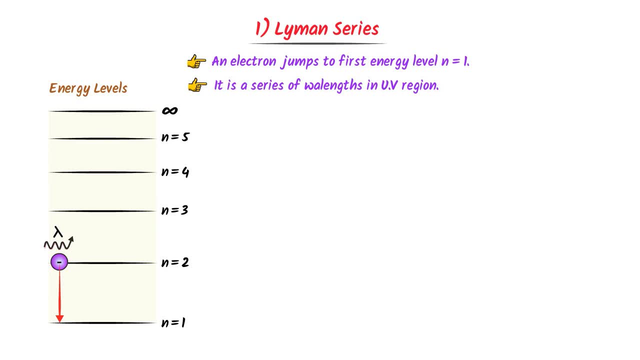 We know that it will emit a specific wavelength. lambda Find its value. We already know the formula 1 upon lambda is equal to rate of zebra, is 1 by 9 minus 1 by 9.. Now the atomic number of hydrogen. 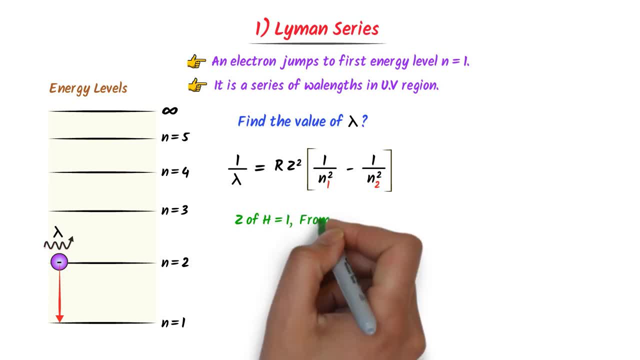 z is equal to 1.. The electron jumps to n is equal to 1. from n is equal to 2. energy level I write: 1 upon lambda is equal to r. n to 1, n to 1 upon 1 squared minus 1 upon 2 squared. 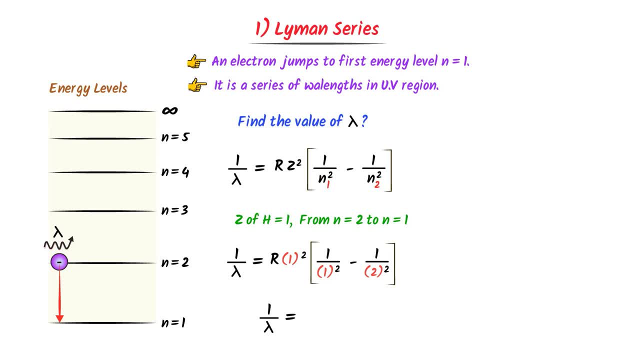 I get. 1 upon lambda is equal to r? n to 3 by 4 r. lambda is equal to 4 upon 3 r. We know that the value of 1 by r is equal to 911 angstrom. I write. lambda is equal to 4 by 3. 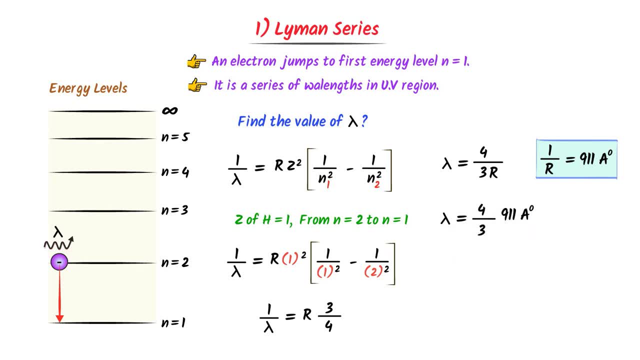 and to 911.. After calculation I get: lambda is equal to 1216 angstrom. Thus the wavelength is 1216 angstrom. If electron jumps from n is equal to to n is equal to 1.. Secondly, let this electron jumps from third energy level. 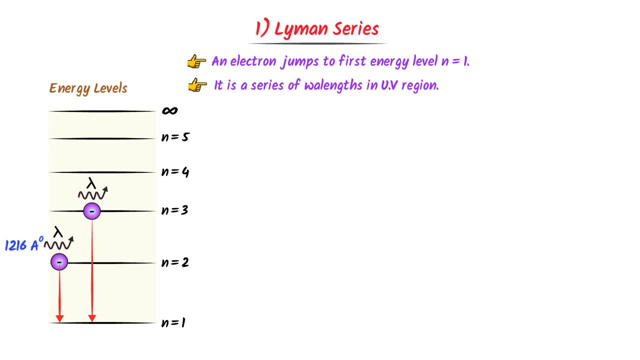 to first energy level, It will emit this wavelength. Find its value. Well, I write the equation: 1 upon lambda is equal to: rate of zebra is 1 by 9 minus 1 by 9.. We know that atomic number of hydrogen is 1.. 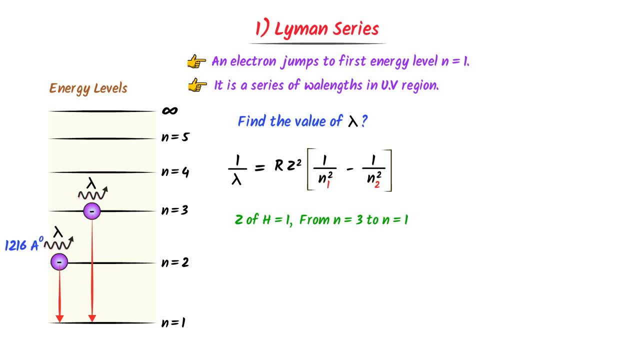 The electron jumps from n is equal to 3 to n is equal to 1. energy level. 1 upon lambda is equal to r n to 1 and to 1 by 1 squared minus 1 by 3 squared, I get: 1 by lambda is equal to r n to 8 by 9.. 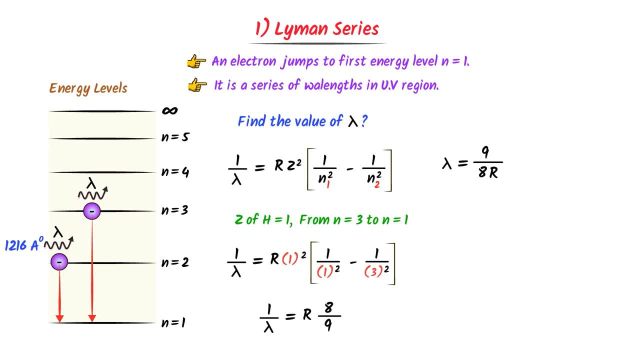 r. lambda is equal to 9 by 8 r. We know that the value of 1 by r is equal to 911 angstrom. I write: lambda is equal to 9 by 8 n to 911.. I get: lambda is equal to 1026 angstrom. 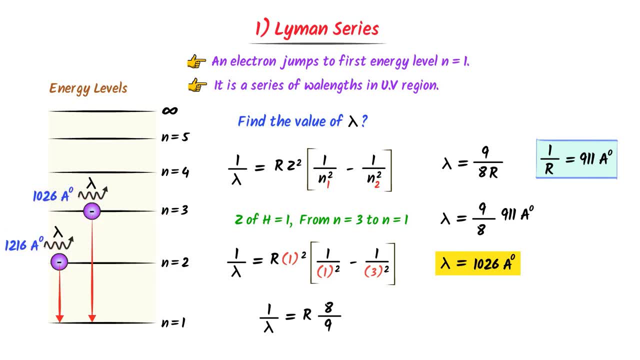 Thus, the wavelength of this radiation is 1026 angstrom. If an electron jumps from n is equal to 3 to n is equal to 1.. Similarly, if an electron jumps from n is equal to 4 to n is equal to 1,. 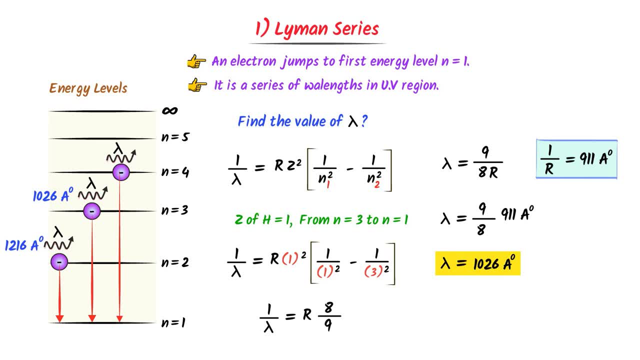 it will emit radiation and its wavelength after calculation will be 972 point at angstrom. If an electron jumps from infinity to n is equal to 1, it will emit radiation and its wavelength after calculation will be 911 angstrom. Just remember that. 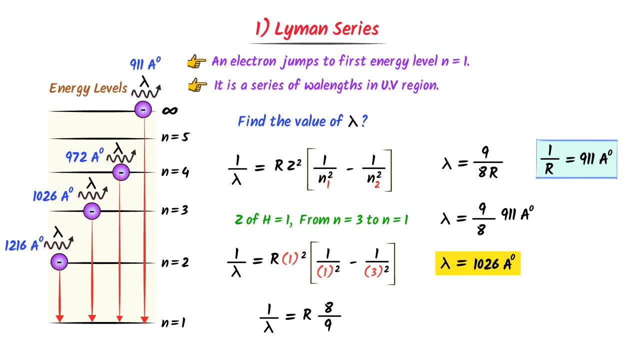 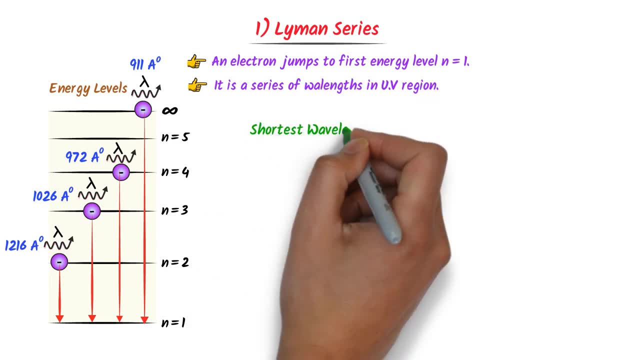 if an electron jumps to first energy level, we will always get Lyman series Here. let me ask you: do you know the shortest wavelength and the longest wavelength of Lyman series? Well, we know that del E is inversely proportional to wavelength. 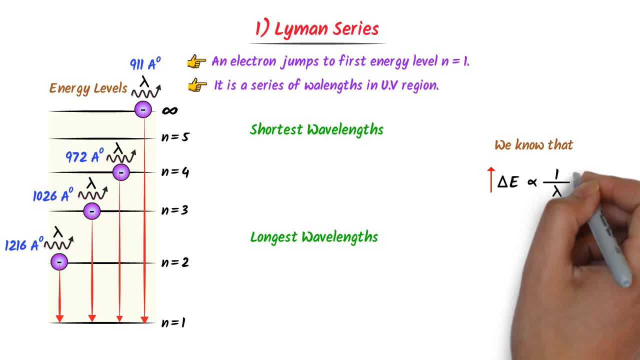 If we increase the energy difference, the wavelength decreases. It means that if an electron jumps from infinity to n is equal to 1, we will get shortest wavelength. For example, we will get 911 angstrom. On the other hand, if an electron jumps from 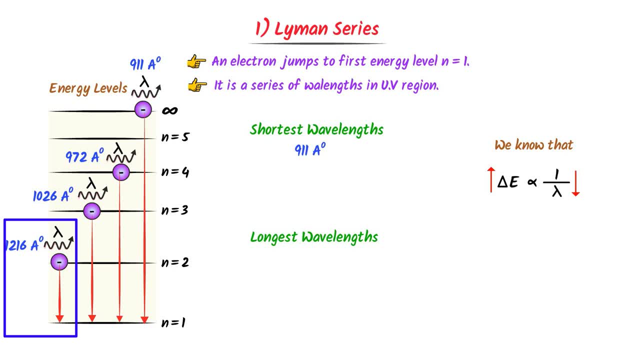 n is equal to 2 to n is equal to 1, we will get longest wavelength of Lyman series. For example, we will get 1216 angstrom. Just remember that for shortest wavelength the energy transition would be maximum, While for longest wavelength 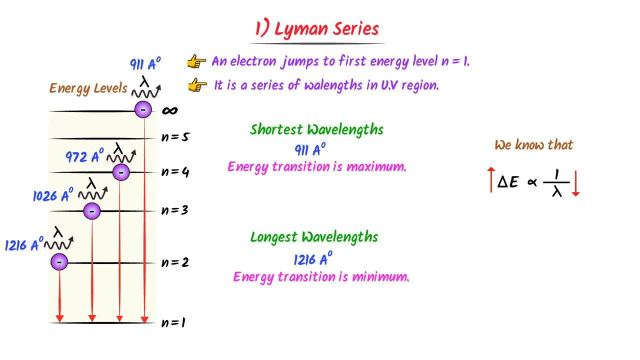 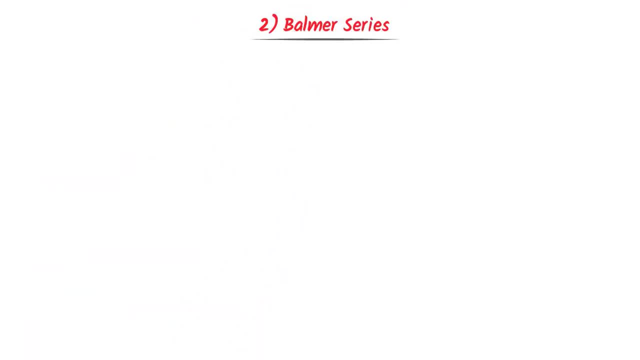 the energy transition would be minimum. Hence note it down, all these important points. Now the second series of atomic spectrum of hydrogen is Balmer series. I write these two important points. Firstly, an electron will always jump to. n is equal to 2 energy level. 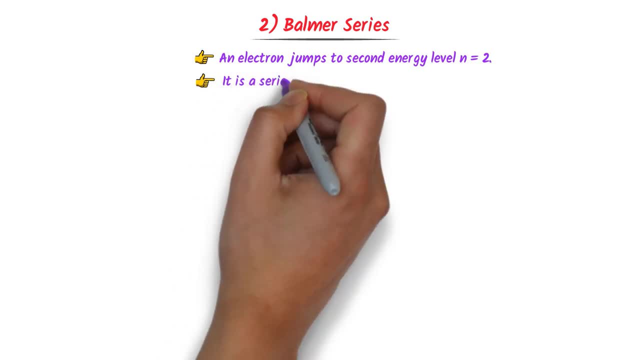 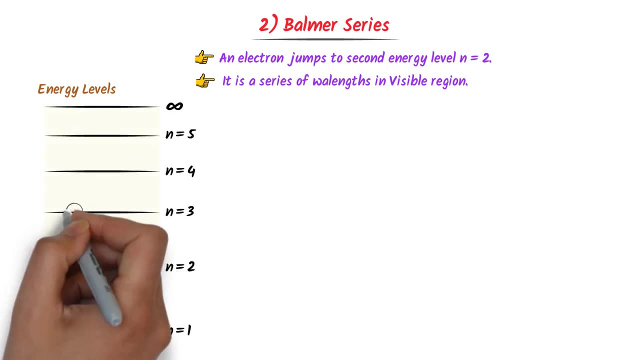 and the Balmer series. Secondly, it is a series of wavelengths and the visible region. Now consider these energy levels. When an electron jumps from n is equal to 3 to n is equal to 2, it will emit this wavelength. 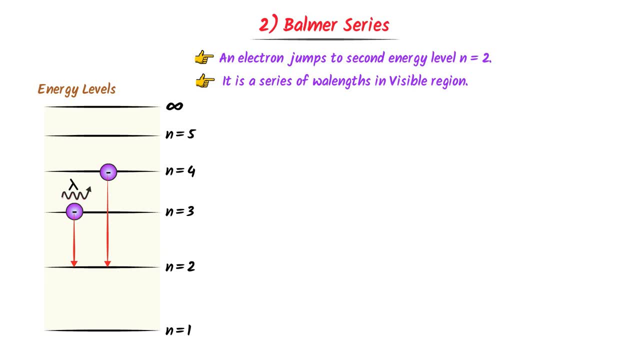 When an electron jumps from n is equal to 4 to n is equal to 2, it will emit this wavelength. Similarly, when an electron jumps from infinity to n is equal to 2, it will emit this wavelength. Now let me ask you. 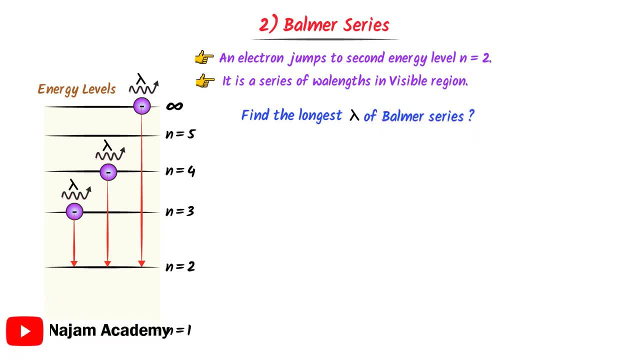 find the longest wavelength of Balmer series. Can you calculate it? Well, we know that for longest wavelength the energy transition must be minimum. That is when an electron jumps from n is equal to 3 to n is equal to 2.. 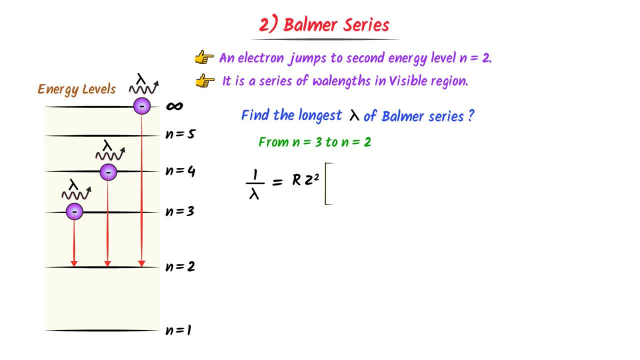 We already know that 1 upon lambda is equal to rate of Zebra, is 1 by 9 minus 1 by 9.. We know that the atomic number of hydrogen is 1 and electron jumps from n is equal to 3 to n is equal to 2.. 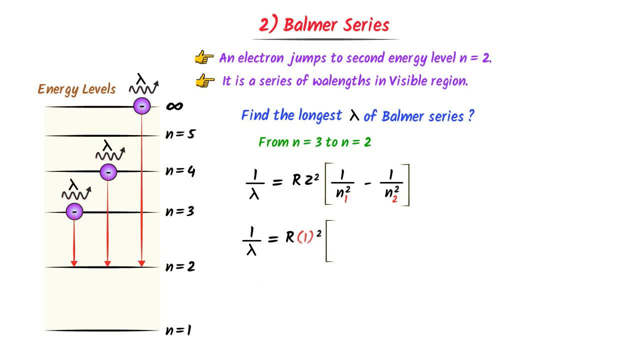 I write: 1 upon lambda is equal to R n to 1. n to 1 upon 2 squared, minus 1.. minus 1 upon 3 squared, After calculation, I get: 1 upon lambda is equal to R. n to 5 by 36. 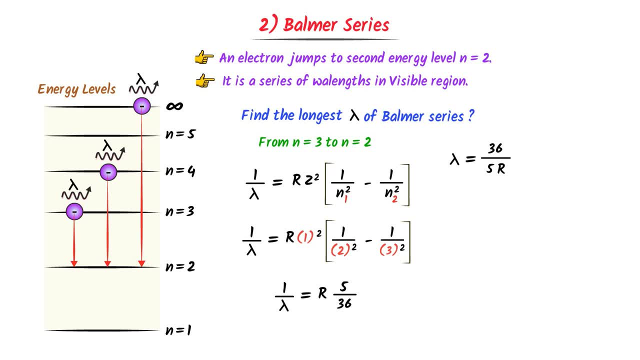 or lambda is equal to 36 by 5 R. The value of 1 by R is 911. angstrom. I write: lambda is equal to 36 by 5 n to 911.. I get: lambda is equal to 6,559. 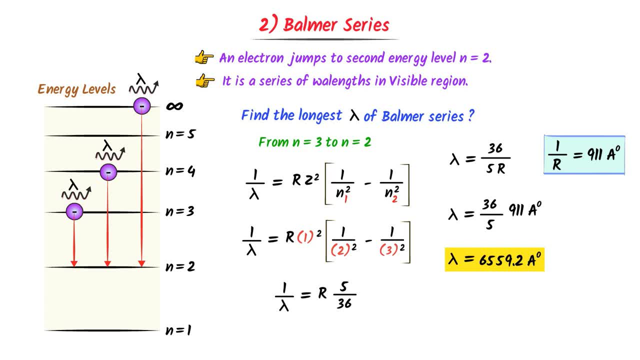 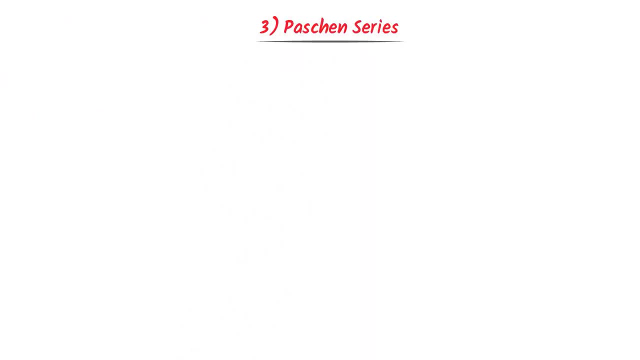 point 2 angstrom. Hence the longest wavelength of Balmer series is 6,559, point 2 angstrom. Thus noted down these important points. Now the third atomic spectrum of hydrogen is Paschen series. As usual, I write these two important points. 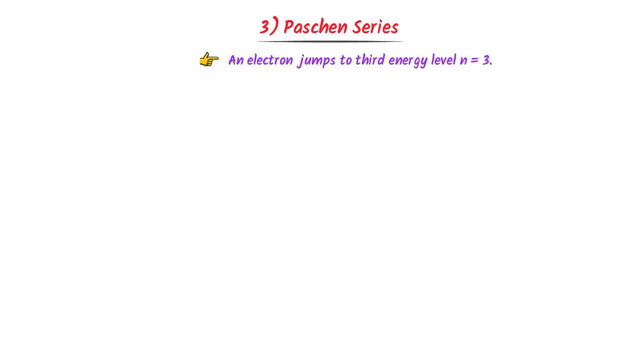 Firstly, an electron jumps to n is equal to 3 in Paschen series. Secondly, it is a series of wavelengths in near infrared region. Now consider these energy levels. When an electron jumps from n is equal to 4 to n is equal to 3,. 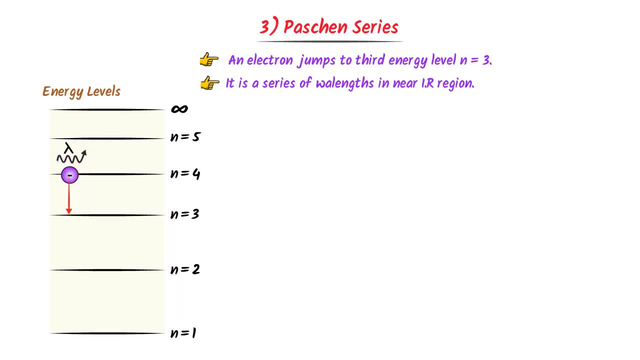 it will emit this wavelength. Secondly, when an electron jumps from n is equal to 5, it will emit this wavelength. Also, when an electron jumps from infinity, it will emit this wavelength. Here let me ask you find the shortest wavelength. 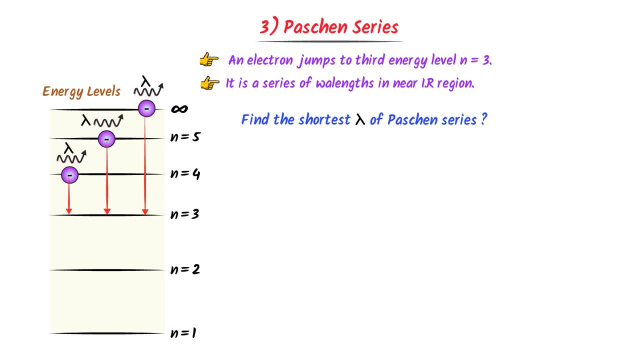 of Paschen series. Pause the video and try to solve it. Well, when an energy transition is maximum, the wavelength would be shortest. I mean, when an electron jumps from infinity to n is equal to 3, we will get the shortest wavelength. 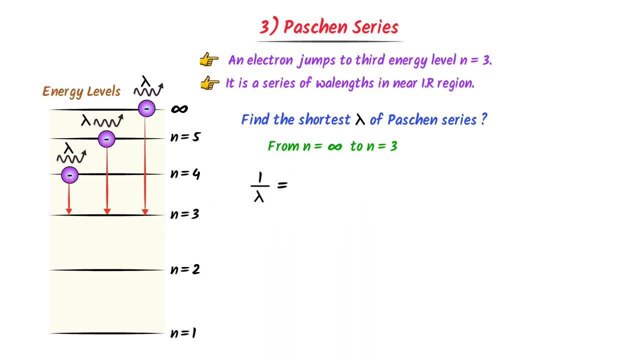 We already know that 1 upon lambda is equal to rate of zebra, is 1 by 9 minus 1 by 9.. r1 by lambda is equal to r into 1, into 1 by 3, squared minus 1 by infinity. 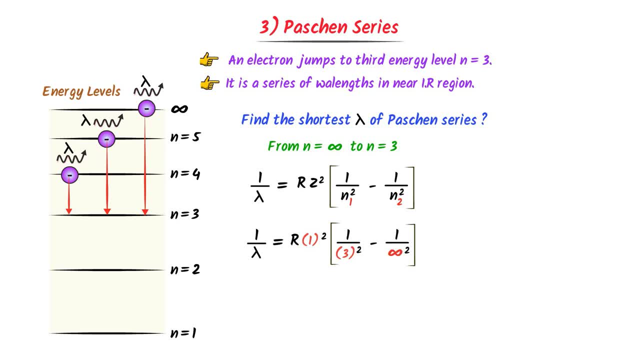 Because the electron is jumping from the infinity, this term is cancelled out. I get. lambda is equal to 8,199 angstrom Hence the shortest wavelength of Paschen series is 8,199 angstrom Hence note it down. 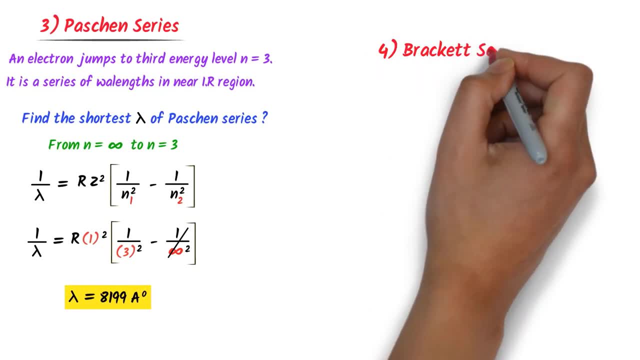 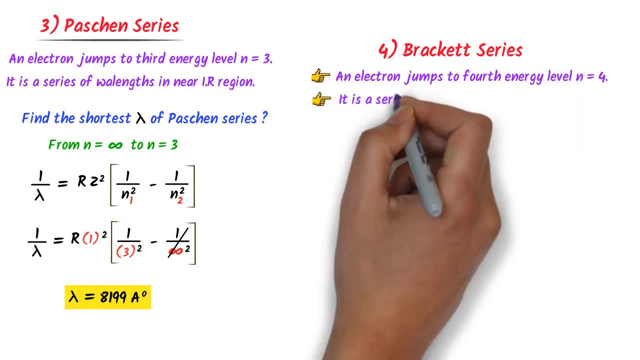 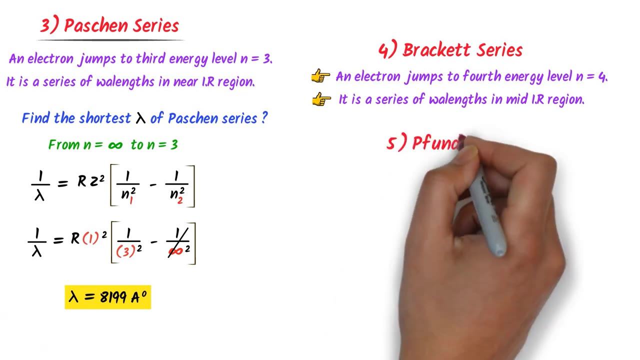 The fifth series of atomic spectrum of hydrogen is Braket series. In this series, an electron jumps to n is equal to 4 energy level. It is a series of wavelengths and mid-infrared region. The sixth series of atomic spectrum of hydrogen is Fern series. 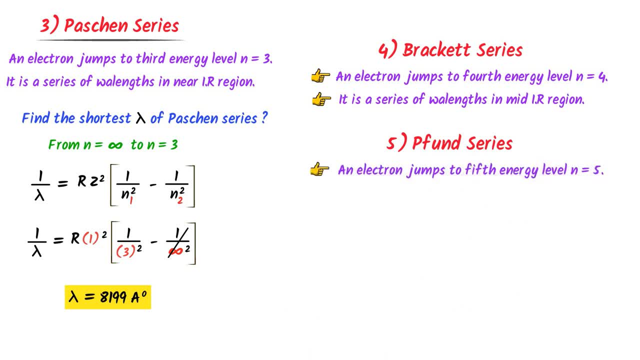 In this series, an electron jumps to. n is equal to 5. It is a series of wavelengths and 4 infrared region. Hence, note it down, all these important points. I hope that you have learnt all about atomic spectrum of hydrogen. 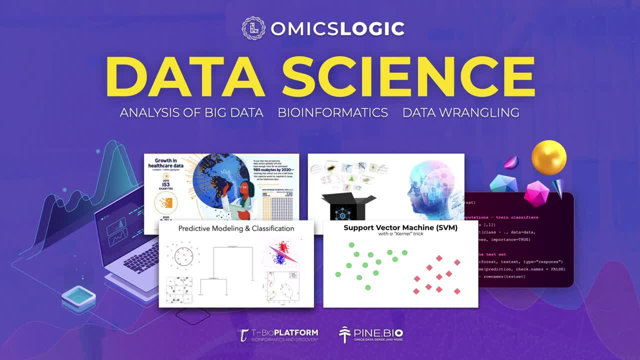 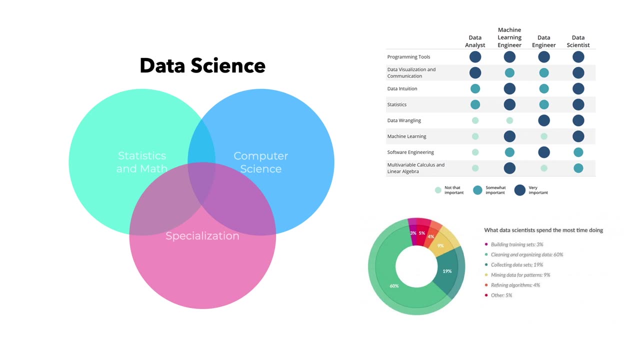 Hello and welcome to OmicsLogic. In this video I will introduce our data science training and explain how you can use various resources to learn about biomedical data analysis, visualization and integration. Data science is a desired profession that brings together diverse skills needed to handle data and turn it into useful information. Some of the highest 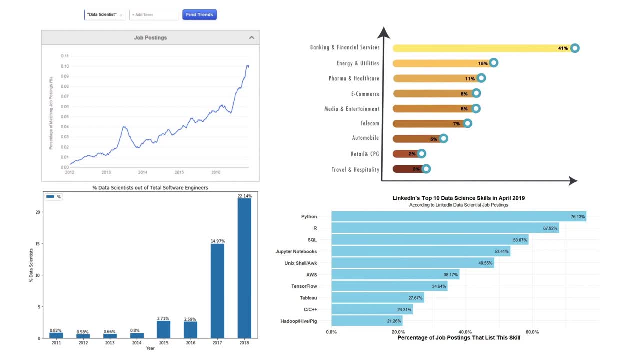 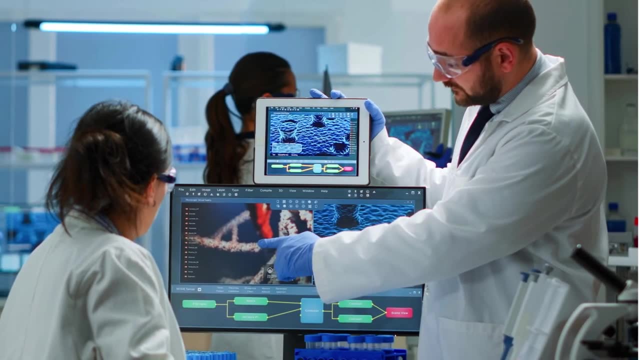 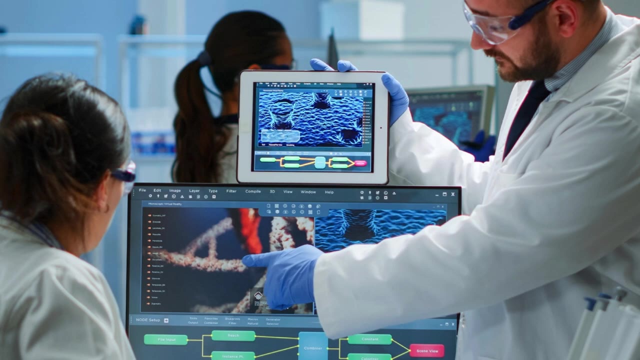 paying and interesting jobs are for data scientists at high-tech companies like Apple, Google and Uber and, more recently, healthcare and biotechnology companies. These industries are relying on scientific discoveries about biology and translating the basic understanding of biological processes into useful insights for many tasks like drug discovery, improved treatment efficacy, as well as early detection. 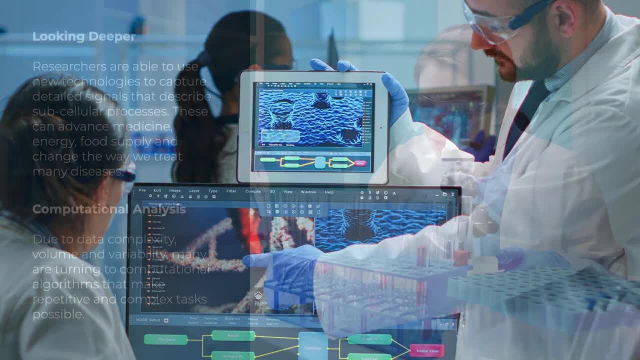 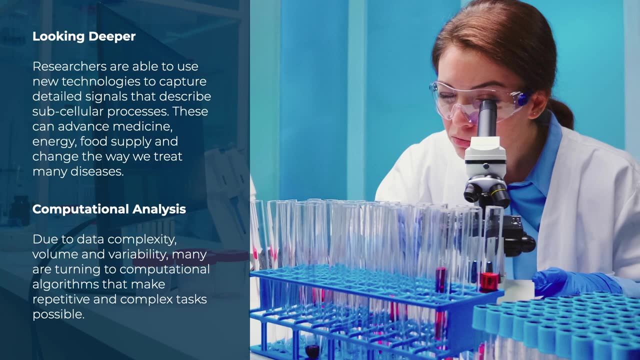 of risks and anticipation of disease progression. These data-intensive applications offer a deeper look at what is going on and require computational analysis skills that today can be used to develop data science techniques. These data-intensive applications offer a deeper look at what's going on and require computational analysis skills that today can be used to develop. 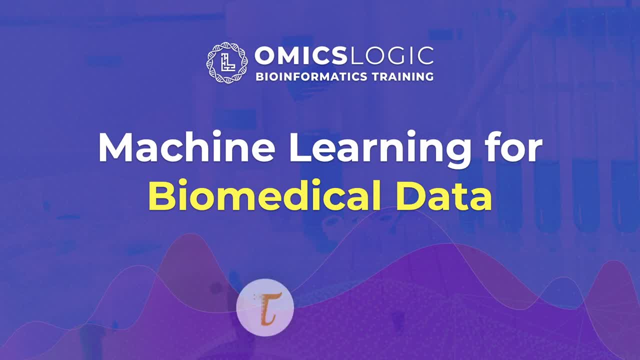 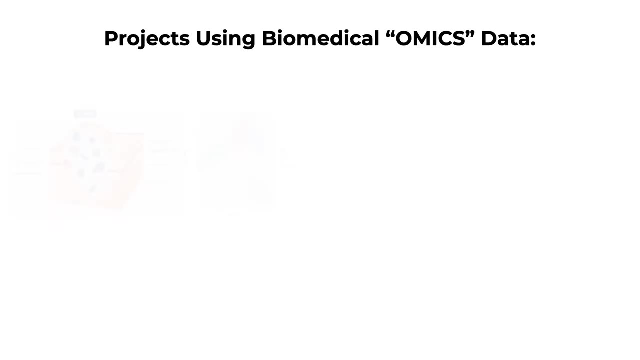 as a tool for addressing and managing data science projects. A major part of our data science be learned by anyone, engineer or biologist. In this program we will cover practical and conceptual aspects of machine learning in application to high throughput biomedical data using various data analysis tools, R and Python. Throughout the course, students will get an 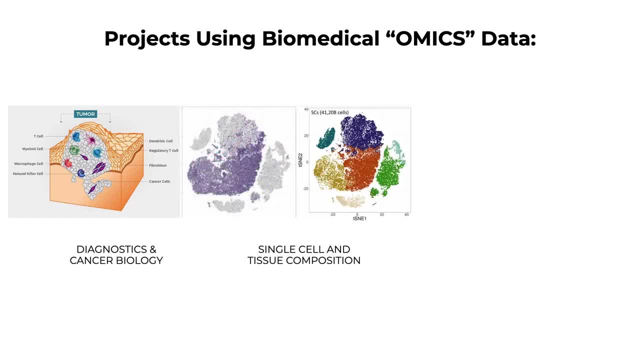 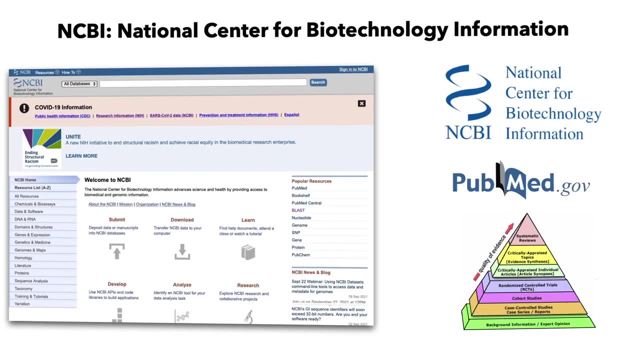 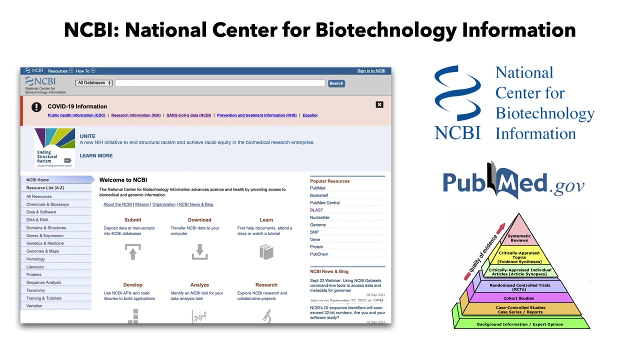 understanding of opportunities and limitations of machine learning in the context of basic and translational biomedical research projects for pre-clinical and clinical applications. Where can you find data on such projects? One repository that we will explore together is maintained by the National Center for Biotechnology Information, or NCBI. 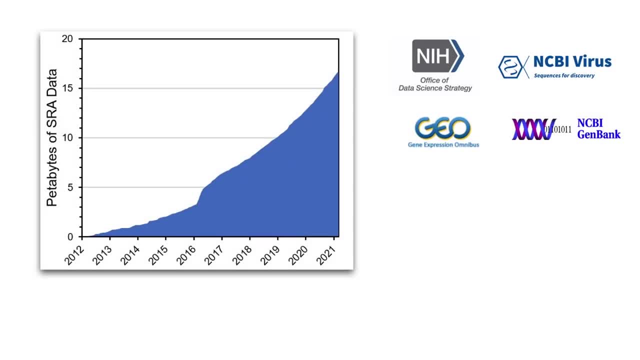 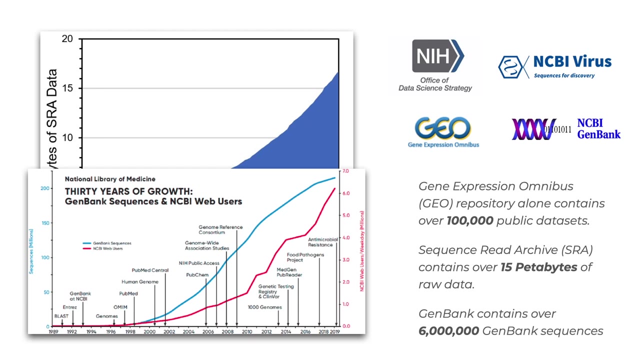 In the past several years, this database has been growing exponentially and today there are over 100,000 publicly available data sets in just one part of the NCBI called GEO, which stands for Gene Expression Omnibus. There are also over 15 petabytes of raw sequence archives.